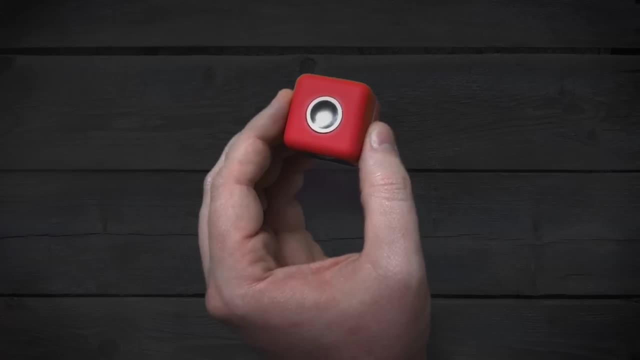 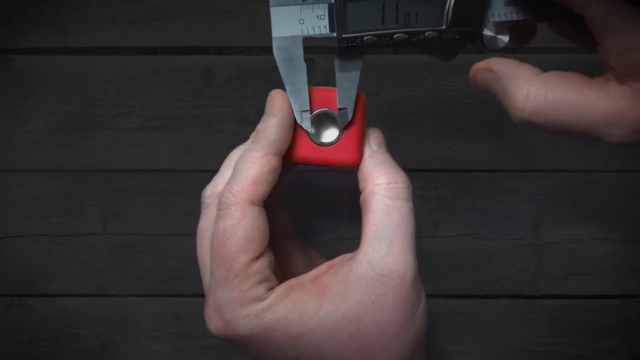 trick and, as usual when I do these sort of math tricks, I'm gonna show you how to do it and then I'll show you why it works after the fact. So, to start with, we're gonna need a couple of pieces of information. We're gonna need to know the 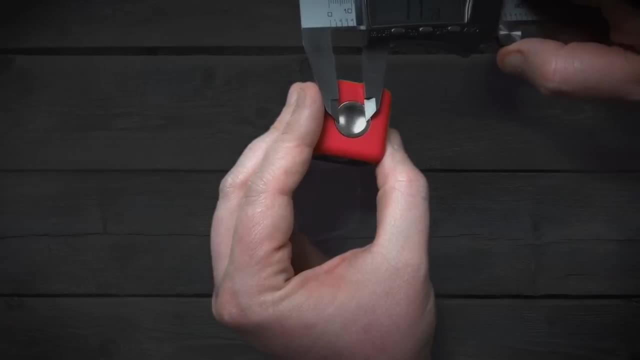 width of our arc, which appears to be, looks like, right around 12 millimeter, or close enough to 12 millimeter. that that's what we're gonna use. We're gonna need to know the depth of our arc, which appears to be basically one point. 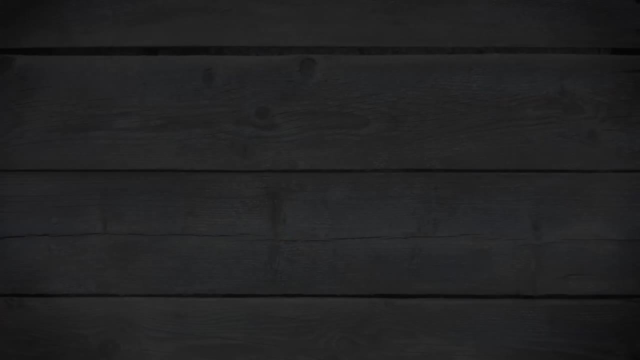 five. So we're gonna use 1.5 and 12 millimeter for our two measurements. I'm assuming this is done in millimeter. we'll find out. So really, what we need to do here is using the length. so say we have the, you know, say this is our arc. 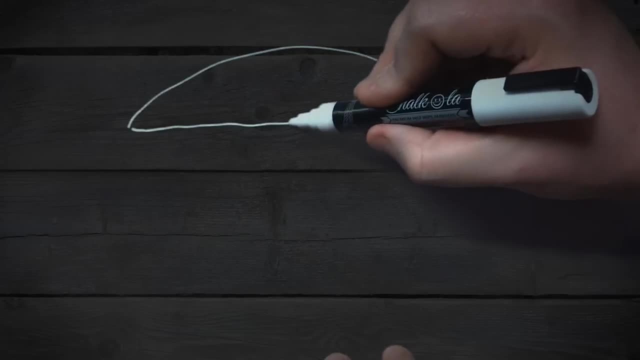 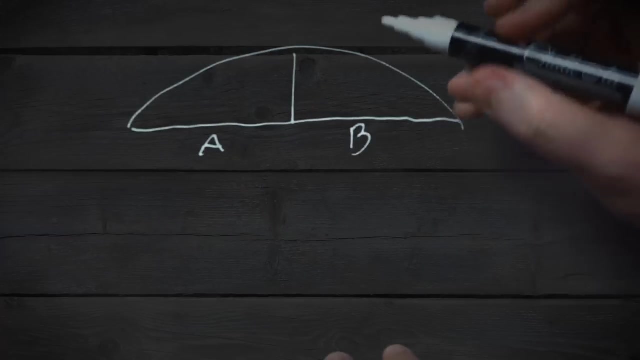 and here we have our length, and here we have our height. Now, if we treat this length as two segments, a part A and a part B, we call the height here C, and we're trying to solve for what we'll call D. Then all you really need to know is that A times B. 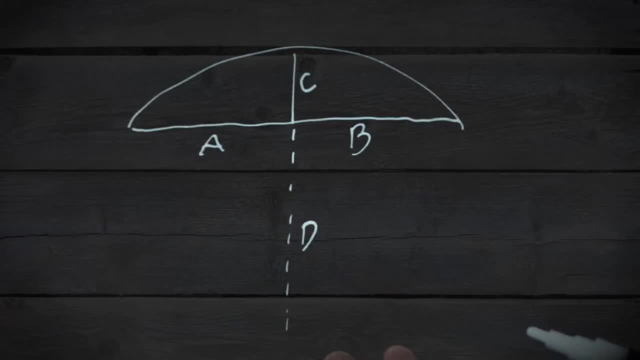 divided by C will equal D. Okay, so in this case we have a total length of 12 millimeter, which makes this 6 and this 6, so 6 squared, we're gonna end up with 36.. We know that this is going to be 36.. 36 divided by our 1.5, which was our height. 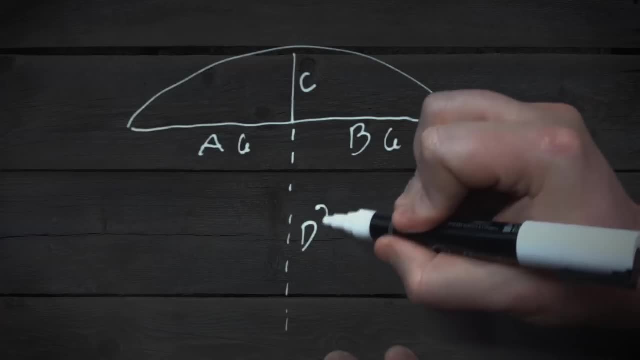 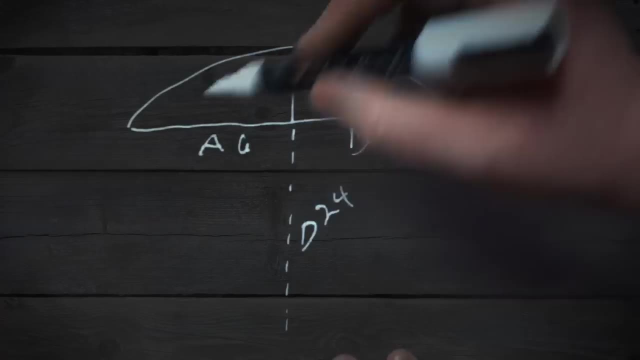 it's gonna be 24, which means this is going to be 4, and then, since this is 1.5, so we know that the diameter of our circle that was used to make that arc is gonna be 24 plus 1.5 or 25.5.. Now, I did this in. 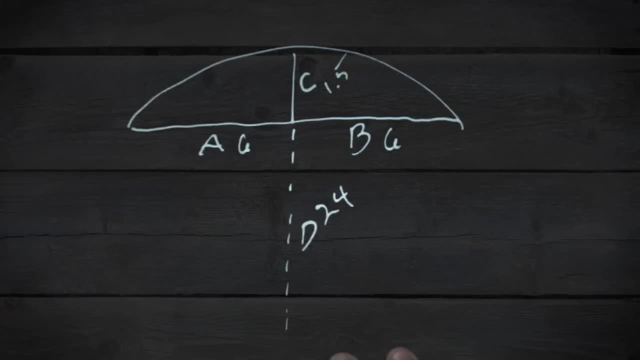 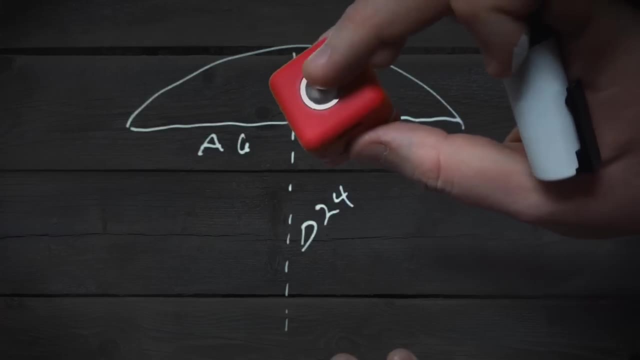 millimeter. 25.4 is one inch in you know directly. so I'm gonna assume this is probably actually one inch, or the metric equivalent of one inch, and that's what I'll use on my dapping block to make a little ball head Now, if you wanted to. 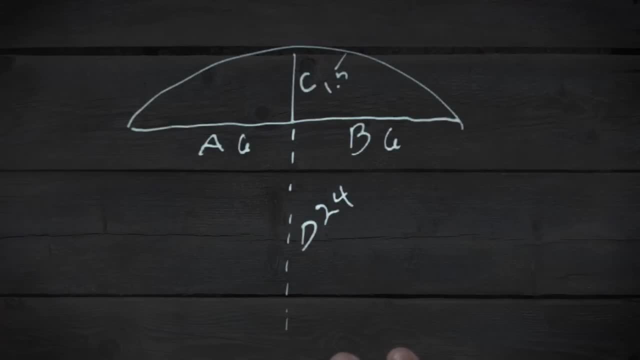 know the actual radius. it would be 24 plus 1.5 divided by 2, and that would give us our actual arc. So just to kind of recap, if you have an arc, any arc, any, you know- doesn't matter how big, if you need to know what size circle was used. 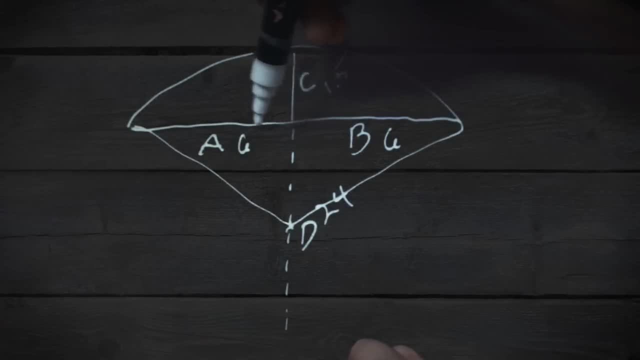 to make that arc, you're gonna need to know of the length divided by 2 squared. so in this case, 12 divided by 2, which is 6. we're gonna just take a and B is same thing, you know. 6 times 6 is 36 divided by our height, which is C in this. 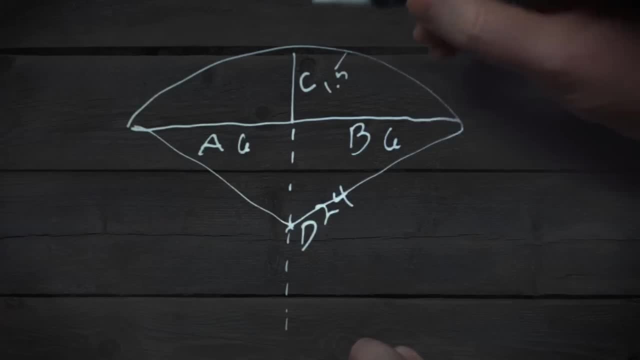 case of 1.5 gives us 24.. 24 plus point five, that's our diameter. 24 plus 1.5, divided by 2, will be our radius. it's really that easy. now, if you want to know why this works, stick around and I will. 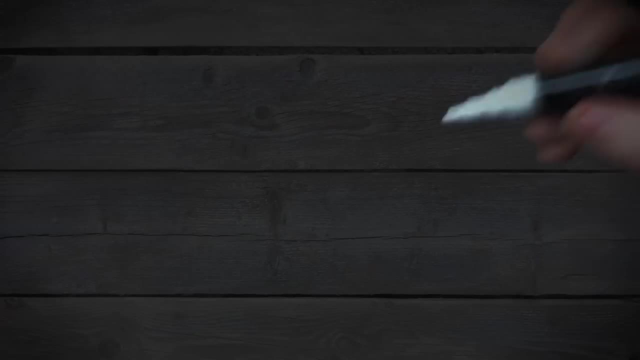 explain it briefly now. the reason this works is because of what's called the intersecting chords theorem, which basically states that if you have a circle and you have any two chords, so a chord being a straight line that connects two points of a circle- any two chords- it could be of any length. now. 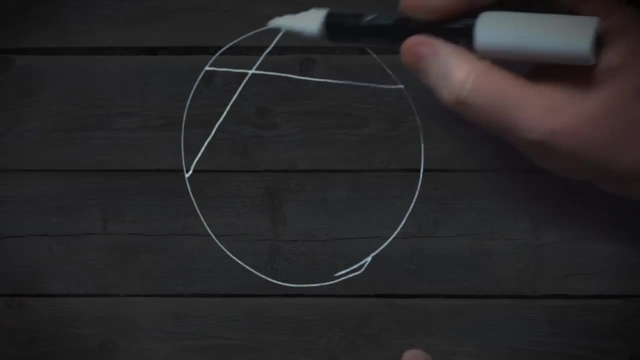 these are obviously- this isn't a very clean circle, but these two- you know chords here- if they intersect, the theorem states that the part a and the part B, the product of those, so if you multiply a times B, will always be equal to C times D. and so in this case, like say a and B equal 36, then C times D. 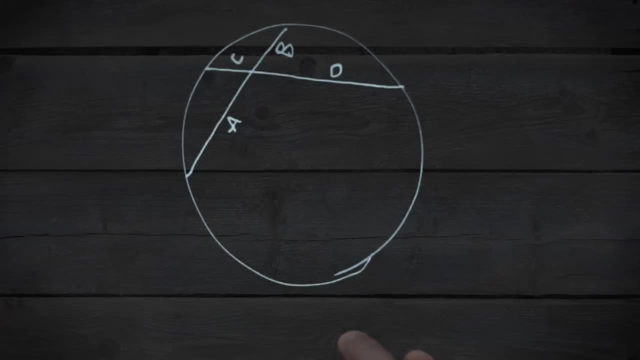 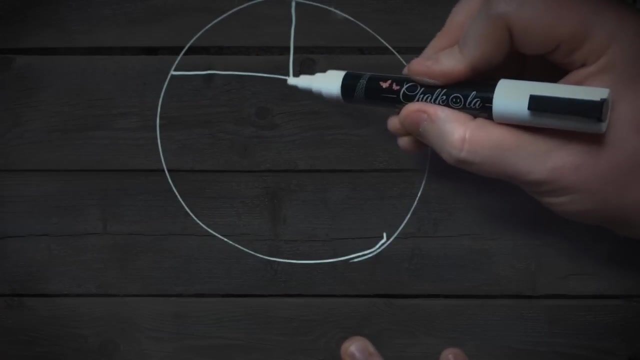 would be equal to 36 too. we know that. you know that's. that's just. we can just take that as a given. so we use that to our advantage by basically pretending that we have a chord and part of a chord okay, and we're trying to solve for the other end. 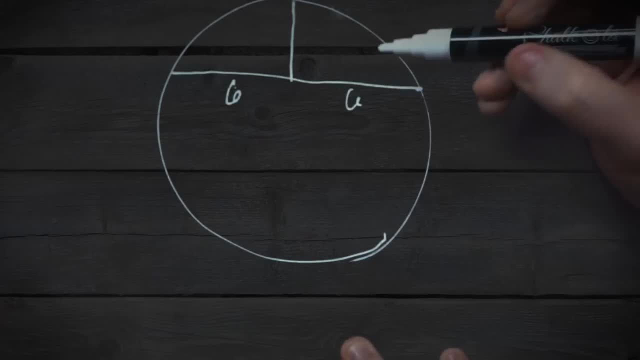 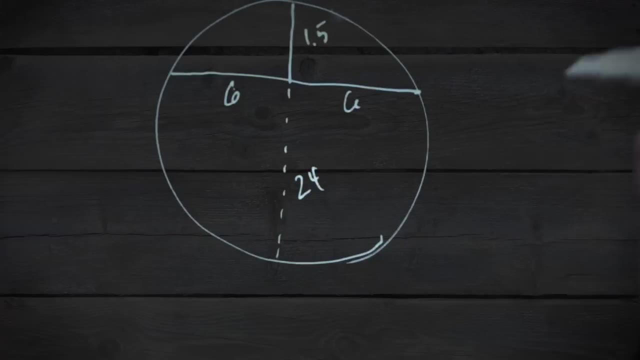 so in this case, we ended up with six and six. six times six equals 36, and this was 1.5, and we're trying to solve this piece, which we now already know is 24. so if you wanted to figure this out algebraically, all you really need to 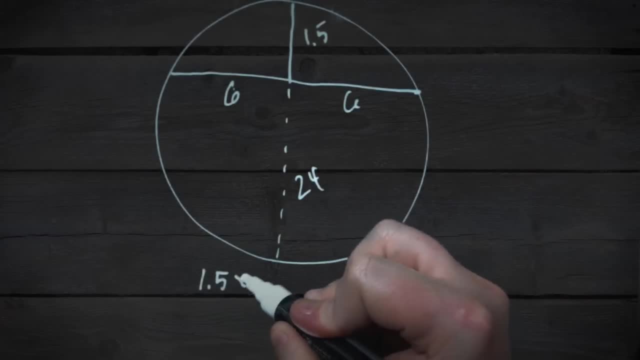 know here is that 1.5 X equals 36. or if you remember your first day of algebra, then X equals 36 over 1.5. so 36 divided by 1.5 will give us our X. in this case, that's our 24. 1.5 plus 24, that's our diameter. divide that by 2 for your. 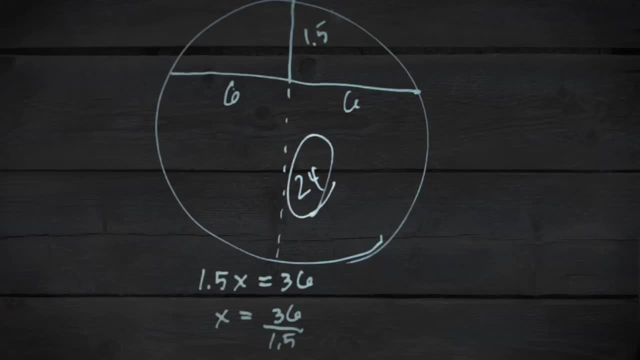 radius, and that's it, so hopefully you find this useful. it's one of those things that doesn't come in handy all the time. there are a lot of great methods for finding the center of a circle and and whatnot, but for like a case like this, you really can't use any of those methods. you.